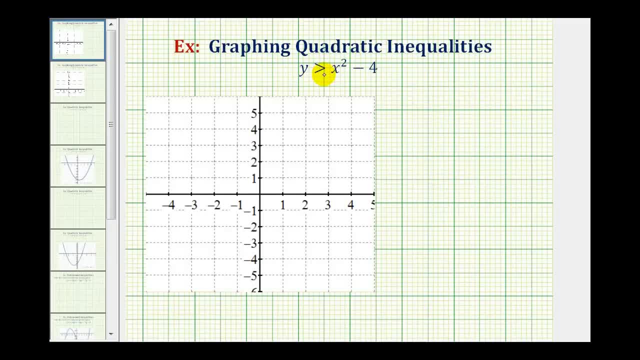 We want to graph the solution to the quadratic inequality. y is greater than x squared minus four on the coordinate plane. The solution to our inequality will be the region on the coordinate plane where the coordinates of all the points in that region will satisfy this inequality. 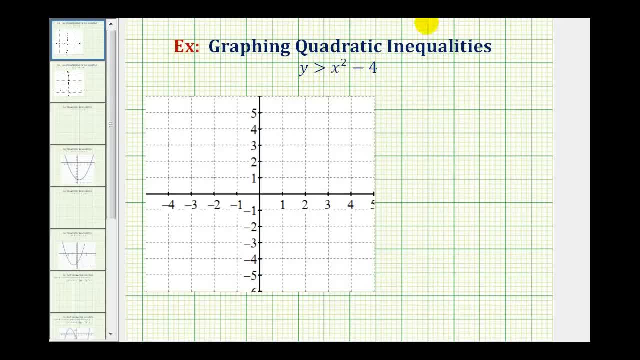 The first step in graphing the solution will be to graph the curve y equals x squared minus four. But because we want the region where y is greater than x squared minus four, the points on y equals x squared minus four will not satisfy this inequality. 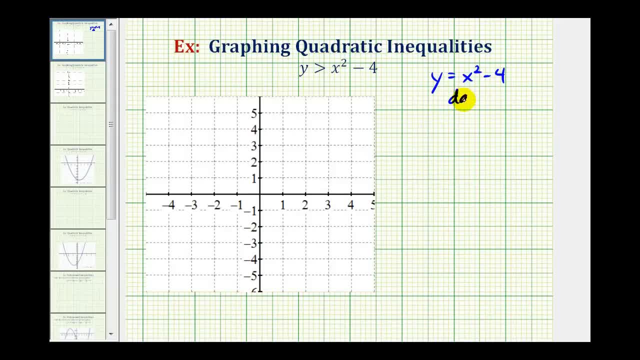 and therefore the graph of our parabola will have to be dashed. If it said y is greater than or equal to x squared minus four, then these points would satisfy the inequality and therefore the graph of our parabola would be solid. 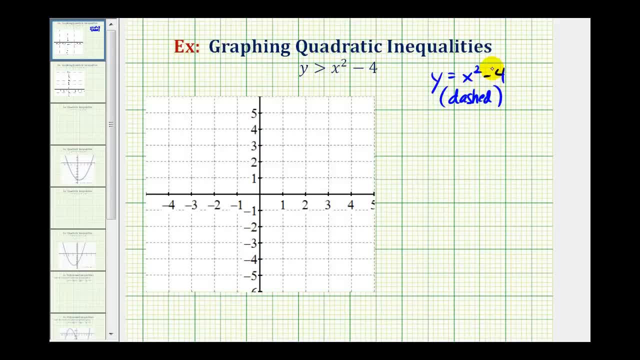 Now we should recognize that this is the graph of: y equals x squared shifted down four. but just in case we don't, we can always make a table of values. Notice: when x is zero, y would be zero squared minus four, or negative four. 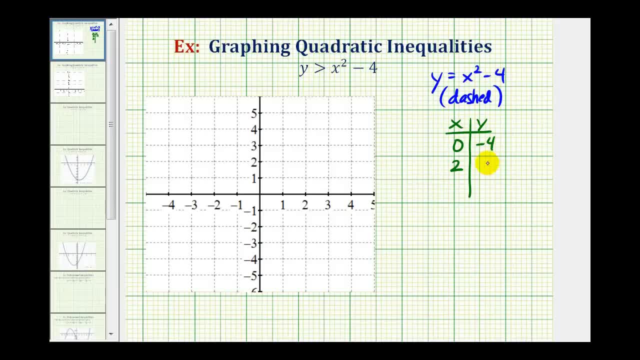 When x is two, y would be two squared minus four. that's zero. And when x is negative, two negative two squared minus four is also zero. So our vertex is the point zero negative four. One. x-intercept is the point two zero. 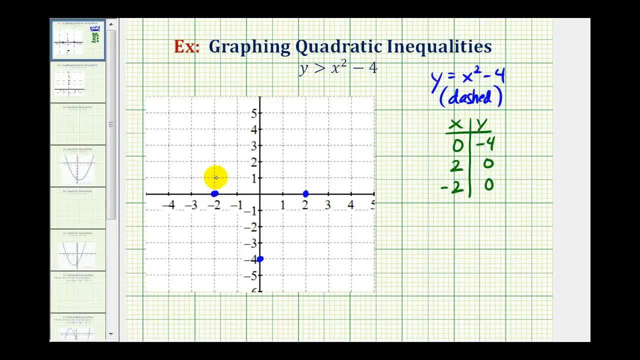 And the other, x-intercept, is zero. One x-intercept is negative, two, zero. Again, because the points on our graph will not satisfy the inequality, we'll make a dashed graph. And now the solution will be the points in the region, inside the parabola or outside the parabola. 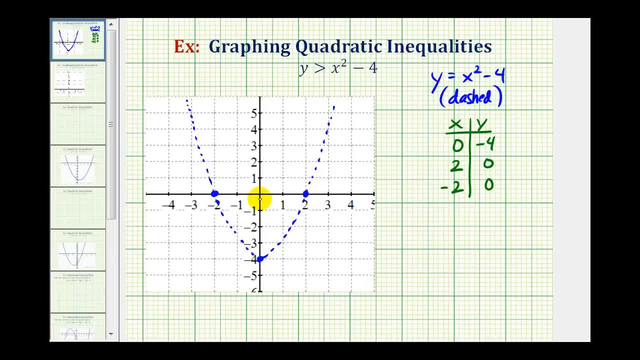 To determine which region to shade, we'll pick a test point and see if the coordinates satisfy the inequality. If it satisfies the inequality, we shade the same region of our test point, And if it's false, we shade the region the test point is not in. 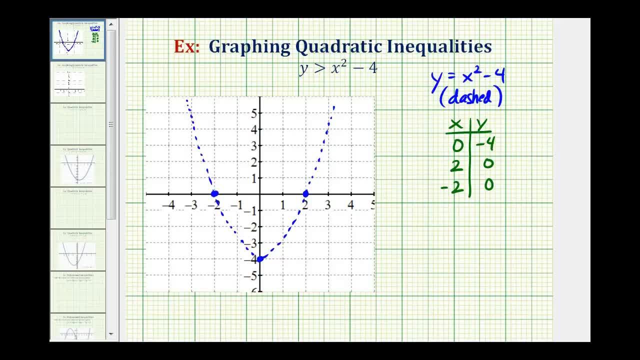 The easiest point to test is the origin, because the coordinates are zero- zero as long as it's not on the graph. If it's on the graph, we'd have to pick a different point. So now we'll test the original inequality using the point zero, zero.